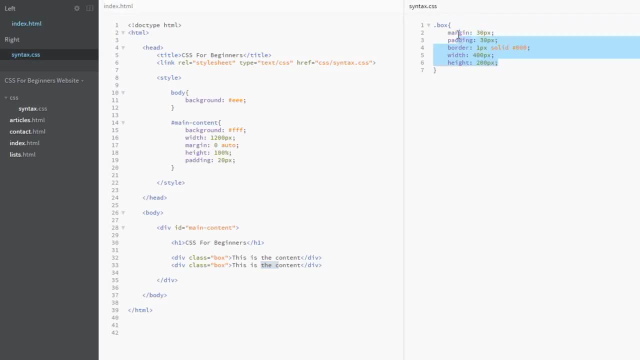 tag. Okay, now I'll give this class of box a few different properties. The first one is the margin of 30 pixels, Remember, that's the external kind of space in between elements. The second one is the padding, which is the internal space, and that's got a padding of 30 pixels. The third one is the border. 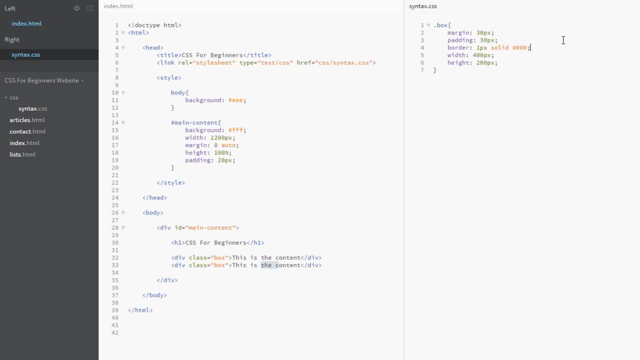 and I'm saying I want that to be solid and one pixel thick and colour of 000 in hex code, which is black, and then I want it to have a width of 400 pixels and a height of 200 pixels. So we've got two of those box classes. 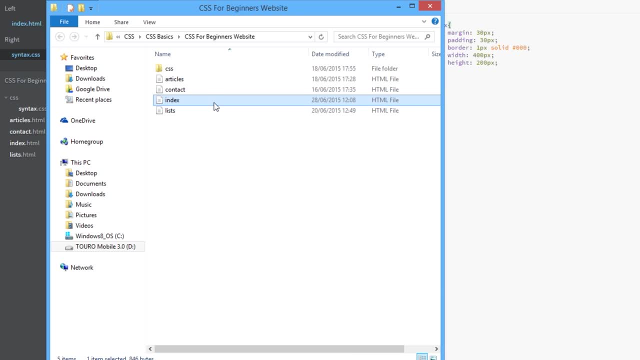 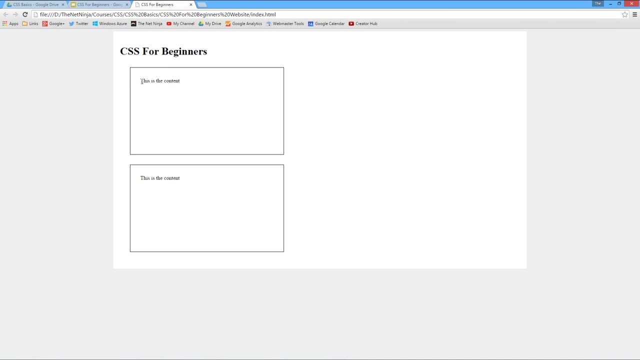 And we're gonna look at this now in a browser. Alright, so you can see, now this is the border, the content in between, and we can't see specifically how big the margins are, how big the padding is, you know the width, that kind of thing. But Google browser, Chrome browser, has this cool thing within. 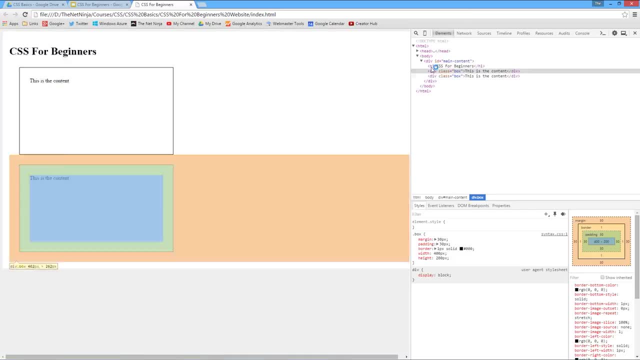 its dev tool. So we go down to inspect element on this and if we hover over one of these elements, then this will show you Deshalb that we're onForever Ontario. we're on this one page now. we're on the blue box in the middle. That is the content: height and width. Okay, so that's. 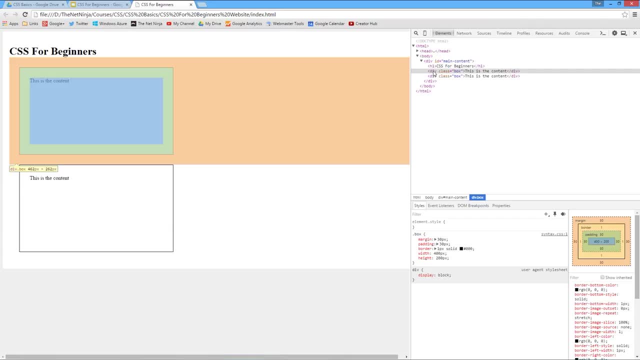 how? I think it was 400 by 200.. Yes, 400 by 200 pixels. That blue debatr represents that space. okay, Now the green colour on there represents the padding and that's 20 pixels. So you can see, all around the blue we've got padding of 20 pixels and then just beyond that is the border. 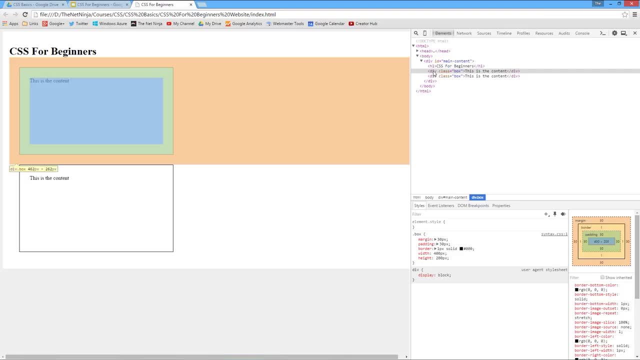 You can see that characterized as a white line. That's one pixel, And then all around that it's a margin of 20 pixels, ipp0, DD pixels. Now you might look at the right hand side of that and say, well, hang on, that's a huge. 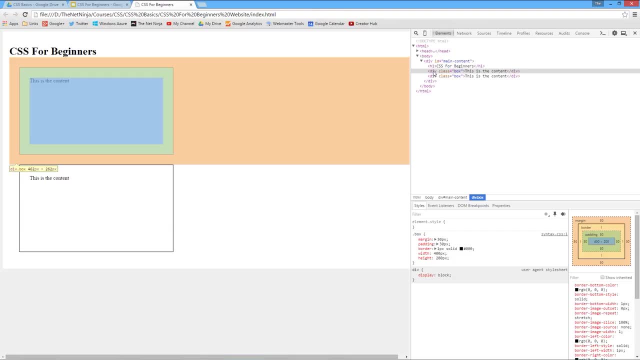 margin on the right hand side, and that's because there's nothing else in that space, so automatically it's applying that margin Because this is a block level element. each block level element occupies it's own space in the document on top of each other, so it's. 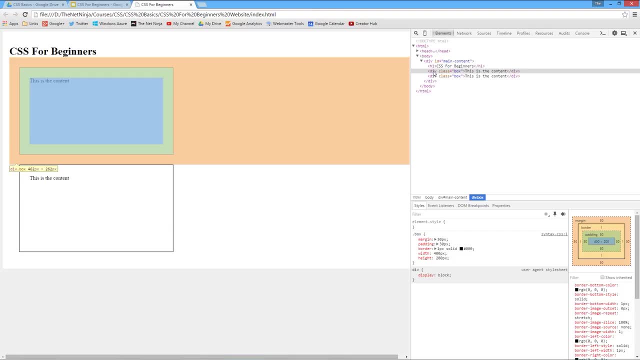 occupying all the space on that row, if you like. So it's using a margin to fill up that space. So that is the box model in action, and Google Chrome also has this cool thing down here. you can see the box model down here in more detail and you can see the main content here. 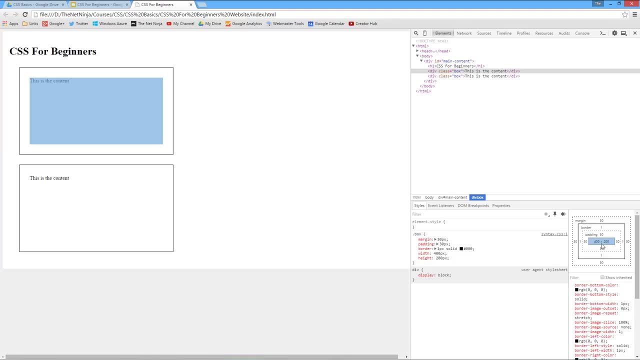 in blue is 400 by 200 pixels. then if I hover over this bit here, it goes green, that's the padding of 30 pixels, the border is 1 pixel thick and then the margin is 30 pixels thick. Now then you may be looking at this and thinking: well, we've got two elements here. 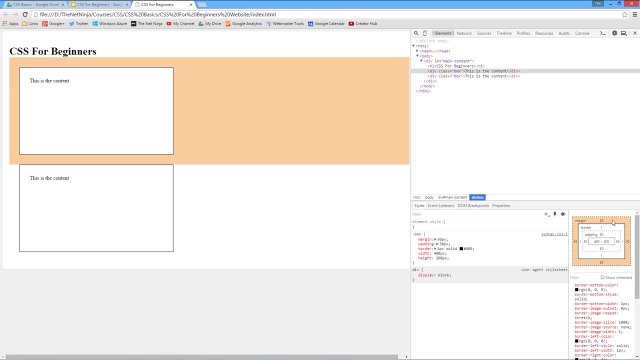 and when I'm hovering over the margin you can see that this space here I'm going to hover over it again. it's 30 pixels in height, that margin. Now we've got 30 pixels on the bottom one as well. how is it we've not got 60 pixels in total between the two elements? 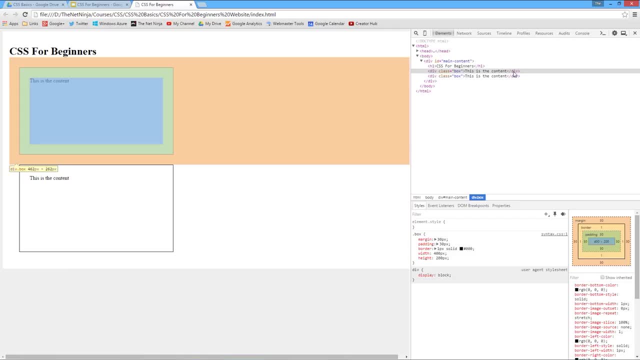 because we've got 30 on this one and 30 on this one. Well, that is a thing called the vertical margin collapse and I'm not going to cover that now. I'm going to do that in a lesson coming up in the future. but essentially, what happens is when you've 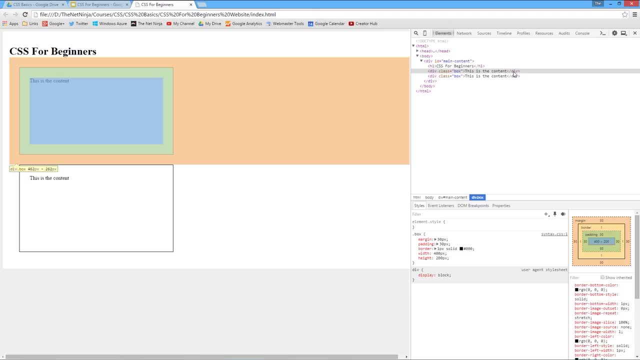 got two vertical margins, they collapse and the higher of the two is taken as the margin. I'll go through this later in more detail, in a different video. I just want to give you a brief overview now. So that's the box model in action, and what I'm going to do now is just see what happens when we take off. 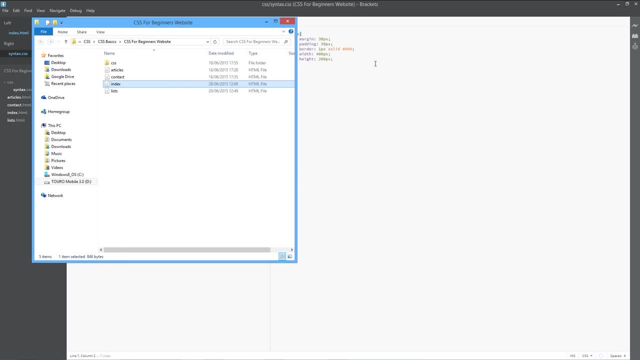 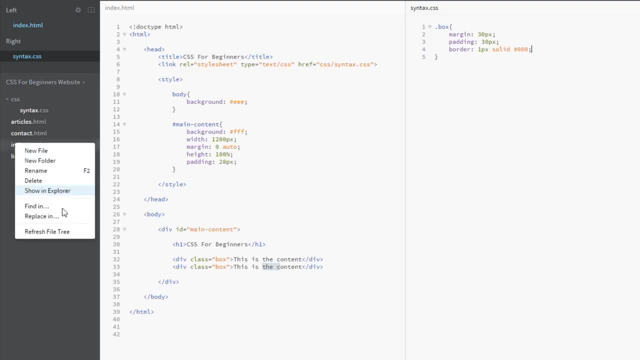 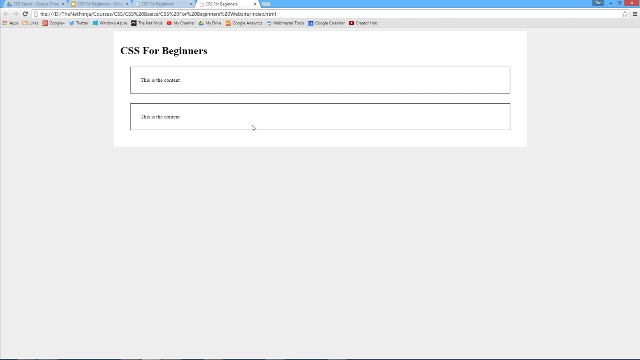 the width properties and the height properties. so let's get these two properties here and delete them. so we're not specifying a width and we're not specifying a height. so let's open this back up in the browser and see what's gone on. all right, so what's happened here is the elements have stretched to, essentially, 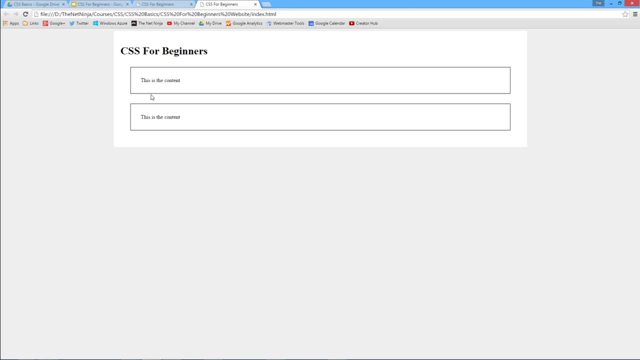 fill the horizontal space here and that's because they're block level elements and essentially every block level element occupies this own, its own space in the document and takes up- if you don't specify the width or height property- a width of the full kind of document width there. So if we 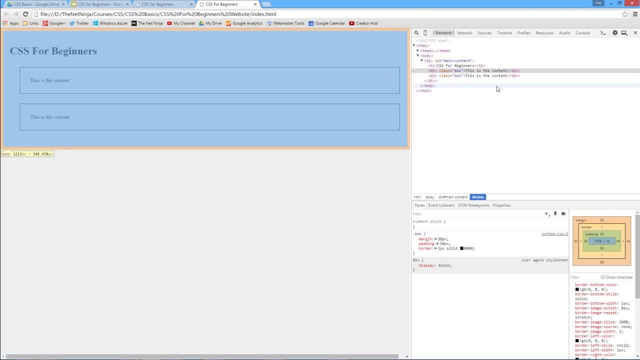 inspect this element again. you can see: now we've got the margin, okay, of 20 pixels. we've got the padding- sorry, 30 pixels, the padding of 30 pixels. then the content is the thin blue strip in the middle. okay, So the height is specified automatically by the height of the 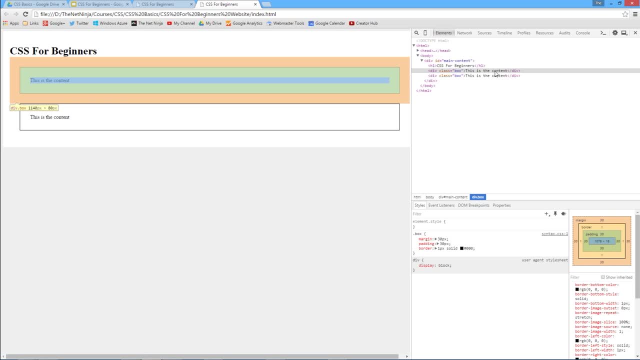 content, which is just the 12 or 14 pixels of height that the P tag is. okay, So they're taking up the full width of the parent element. okay, So that's what happens when you don't specify a width. Now, this is not to be confused with putting width 100%, because that will be slightly. 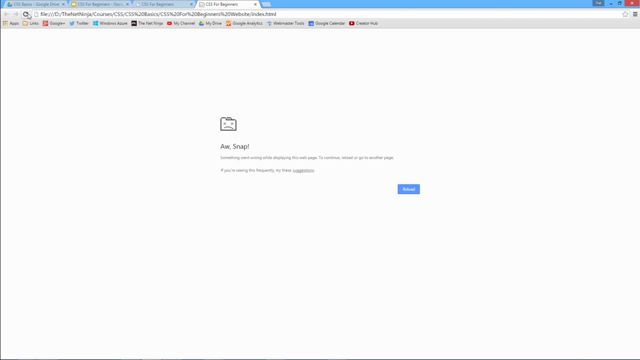 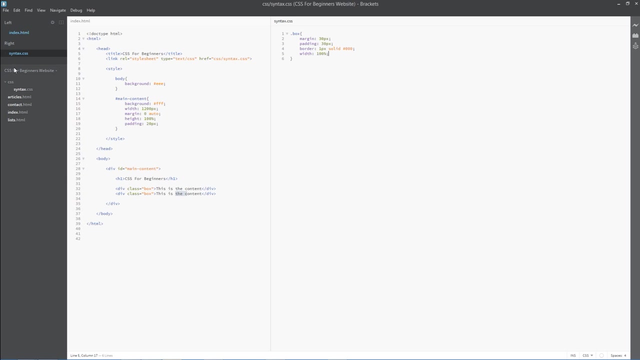 different and I'll show you what I mean. okay, Although that's oops, although this here is essentially occupying 100% of this width. here, apart from the margin which you specified, if we put specifically a width of 100%, you would expect that to be the same right? 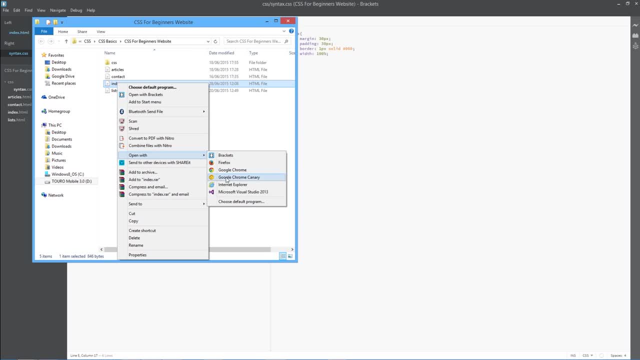 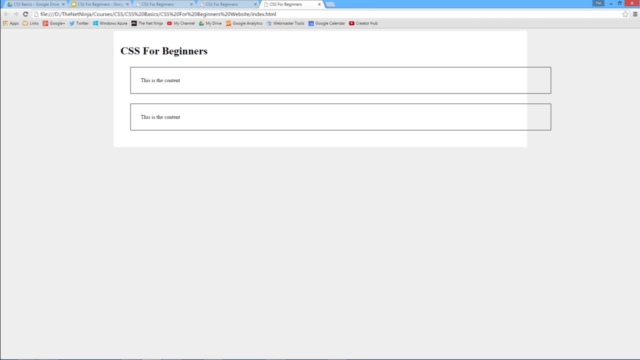 Let's view it in a browser and see what happens then. Okay, now you can see it's gone over and you might be sitting there thinking: well, what you know? I've specified a width of 100%. what the hell's happening here? 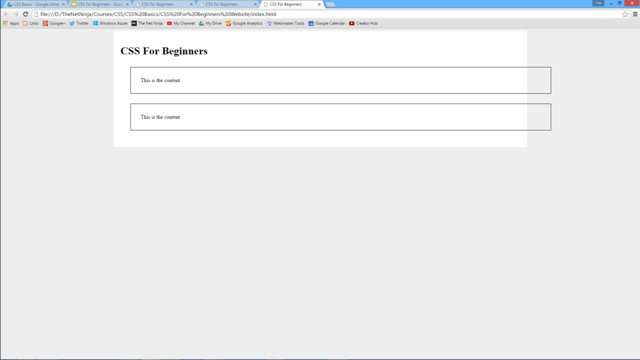 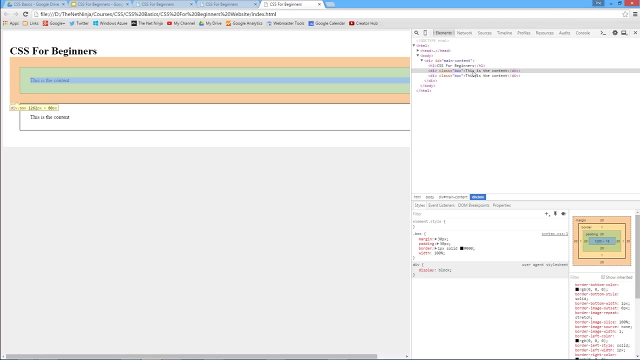 And this is what a lot of designers start out doing when they first start with CSS. They get confused with the box model, and the reason it's doing this is because this width here, if we right-click this blue width here, is giving itself a width of 100%. okay, So just the blue bit. 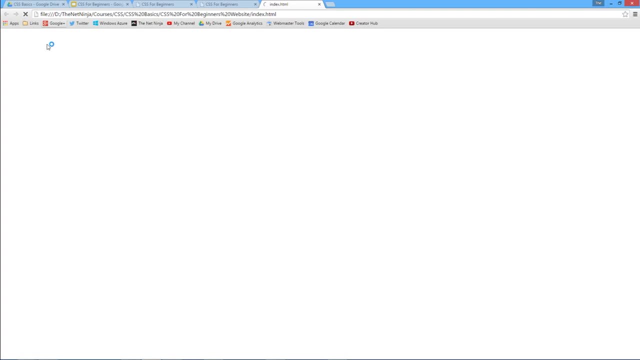 okay, And 100% would be. oops, all of this area here, right, All of this parent element width. So it's giving itself that full 100%. Now, on top of that, it's got the padding of 30 pixels, the border of one pixel and the margin of 30 pixels as well. 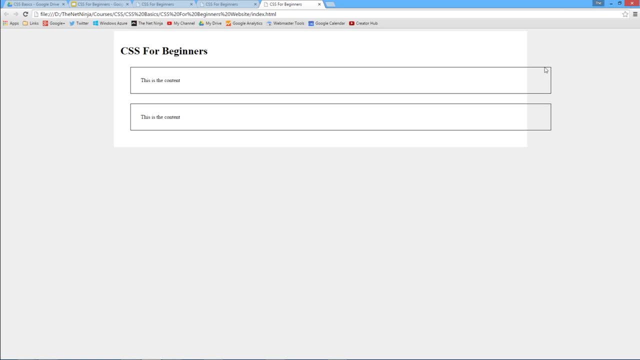 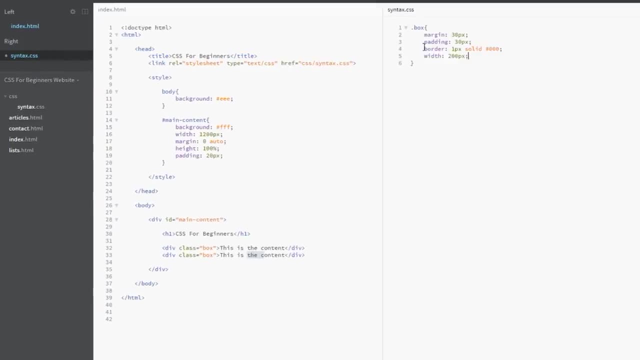 Okay, so it's actually 100%, plus all of that other stuff which is causing it to overflow here. All right, so when we say width 200 pixels, the overall width is not 200 pixels, That's just the width of that little blue bit in the middle, the actual content. 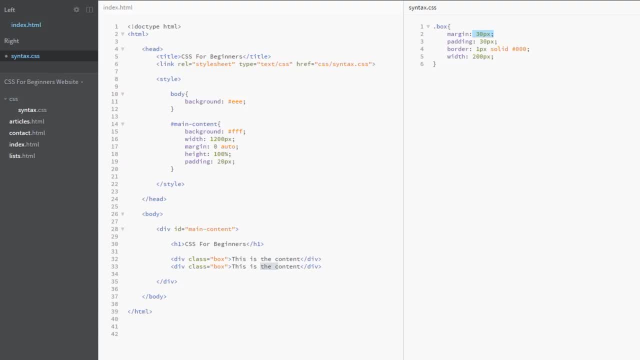 On top of that we've got 30 pixels on each side of margin, So 30%: 30 pixels on the left, 30 pixels on the right, and then we've got padding of 30 pixels on the left and 30 pixels on the right. 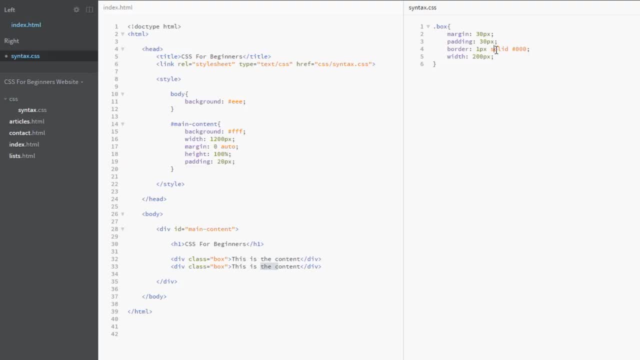 and then we've got this border of one pixel on the left and one pixel on the right, So in total it's essentially 200 in width plus 30 on the left margin, 30 on the right margin, plus 30 on the left padding, plus 30 on the right padding, plus one pixel border on the left.